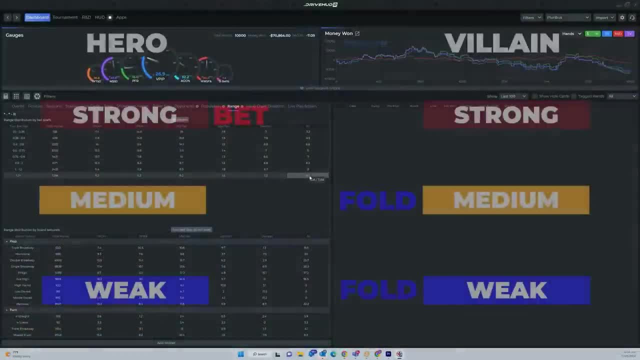 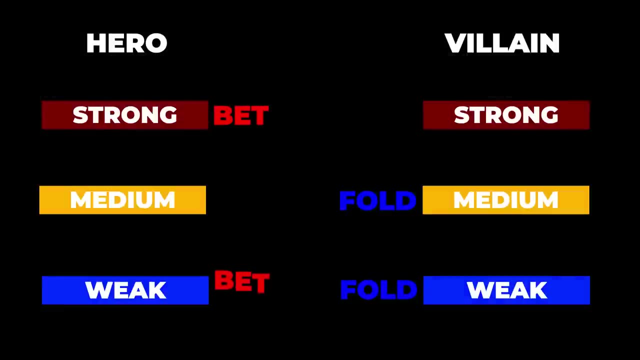 betting strong hands is even easier through the use of heads up displays. So in order to induce our opponents to call our bets when we're holding a strong hand, we need to also sometimes bet with our weak hands, also known as bluffs, And bluffing also has the extra potential benefit of getting. 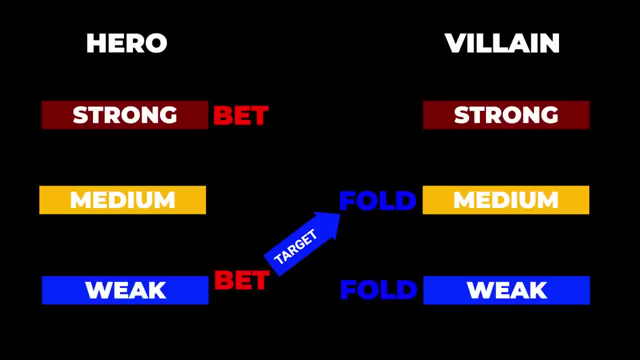 our opponent to fold a better hand. But if you've played poker for a while, you've probably noticed that you will typically have a weak hand much more often than you'll have a strong hand. This means that you can't just bluff every time you're holding a weak hand, or else your discerning 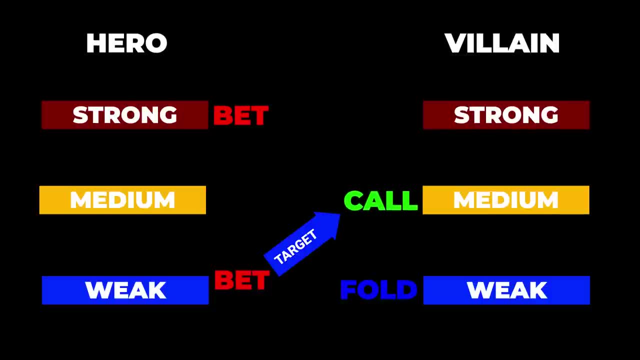 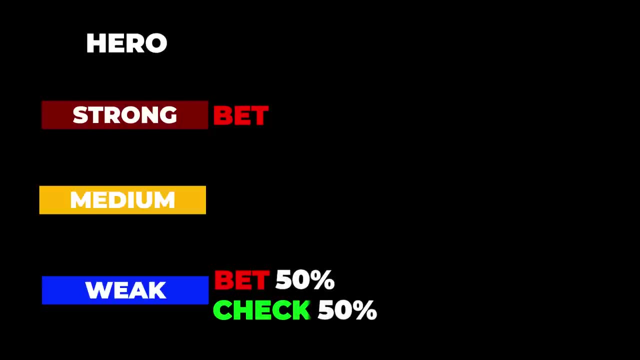 opponents will catch on to this and start taking stands by calling down lighter. So the next question is: how do you decide when to bluff and when not to bluff? Well, you could just flip a coin, and that strategy would probably actually be okay. but there's an even better way You can. 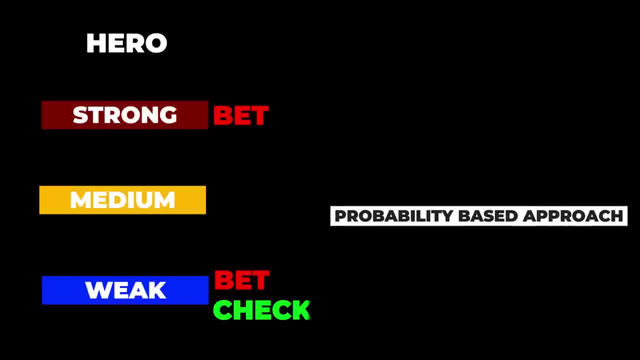 differentiate between your weak hands by their specific characteristics or micro attributes. This is the way you can bluff: when you're holding a weak hand or when you're holding a strong hand. This means that you can't just bluff every time you're holding a weak hand or else your discerning 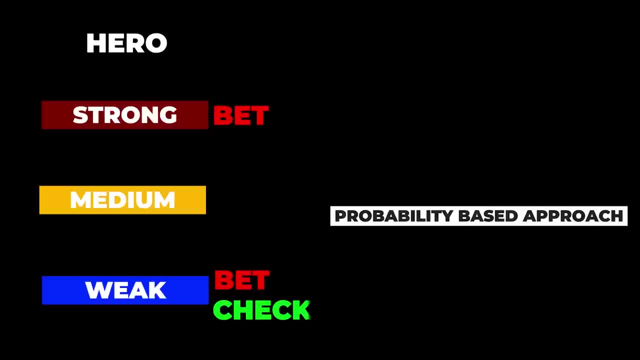 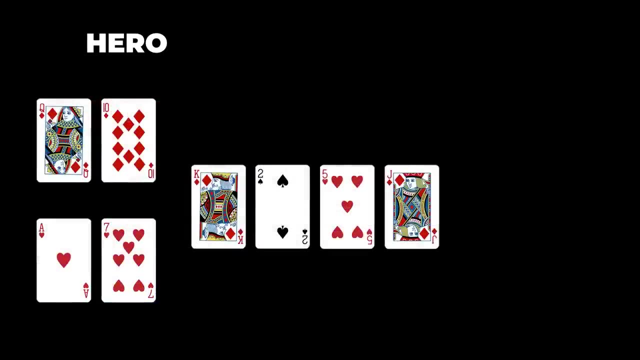 opponent will catch on to this and start taking stands by calling down lighter. This may include deciding to bluff with a good draw, which we refer to as incremental equity, but choosing not to bluff with pure air. For example, on this turn, we could decide to bluff if we're holding queen ten of 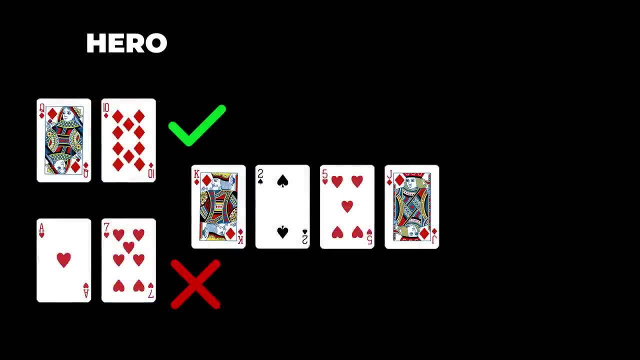 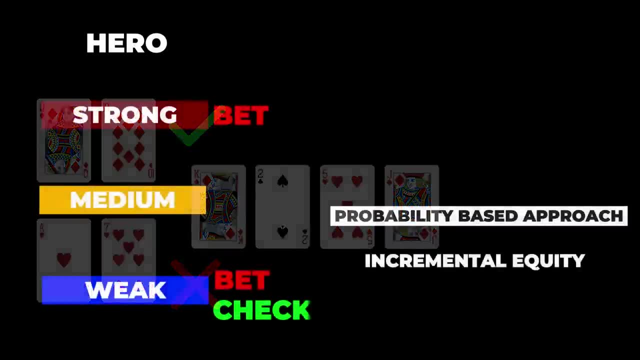 diamonds, but choose to just give up if we're holding a seven of hearts, because we have a much higher chance to hit a big hand and win a big pot with the former due to its incremental equity. We can also choose to bluff when our particular holding makes it more likely that villain will. 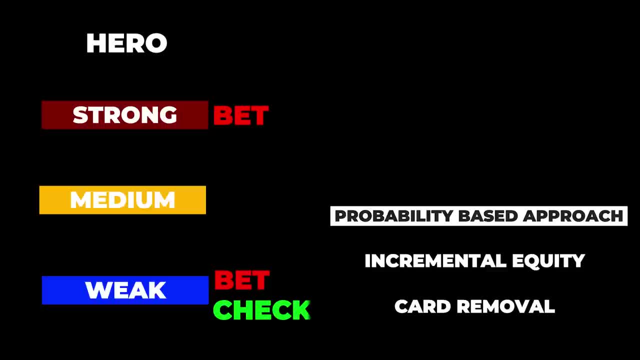 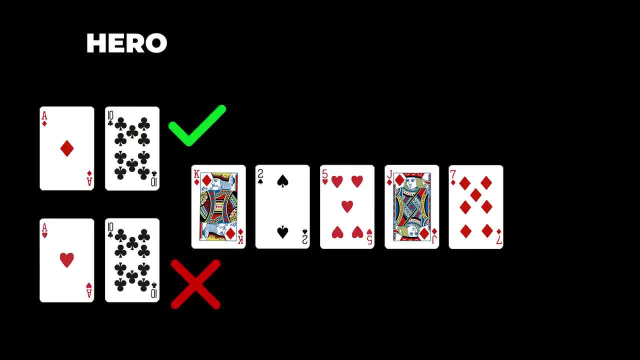 fold from a probability standpoint, which we refer to as card removal. So, on this river, we may choose to bluff with ace of diamonds- ten of clubs- but choose to give up with ace of hearts- ten of clubs. because when we're holding the ace, 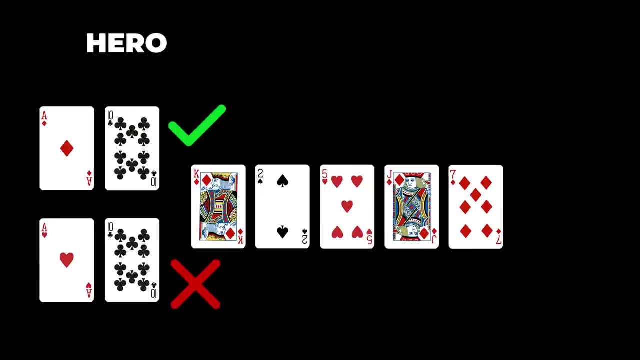 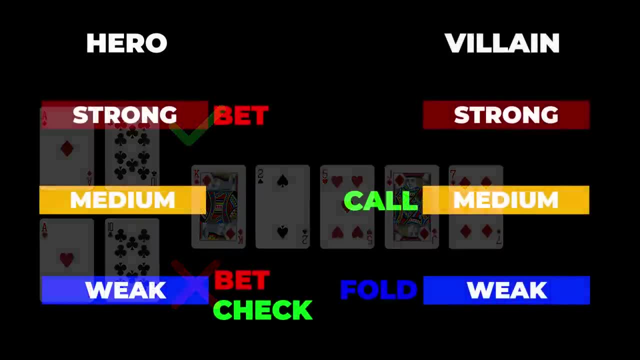 of diamonds, it makes it impossible for our opponent to have the nut flush, which in turn increases the probability that we'll get a fold due to our hand's card removal effects. When you balance betting strong and weak hands in this way, it puts villain in a predicament. 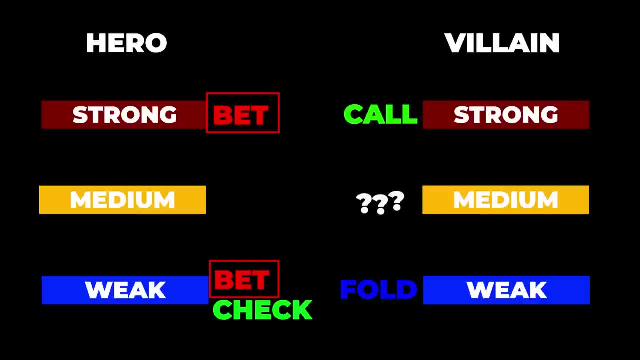 If he has the nuts, then defending is easy. But what about his medium hands, such as second and lower pairs and perhaps strong ace highs? If hero only bets strong hands, then villain can comfortably just fold all his medium hands. and if hero bets all his weak hands, villain can just 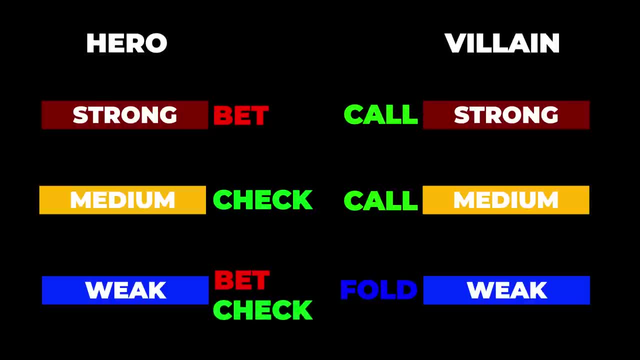 comfortably call all his medium hands. But if hero starts balancing his bets among strong and weak hands, then villain is forced to call some medium hands and fold others. If he doesn't, then hero would be able to readjust by either under or over bluffing. 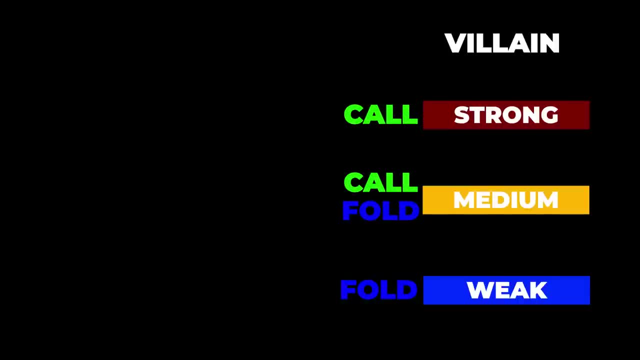 So how does villain decide which medium hands to call and which to fold? Well, again, he could just flip a coin. but, similar to the bluffing situation, villain can improve his chances for calling or folding correctly by choosing hands that have positive incremental equity or card. 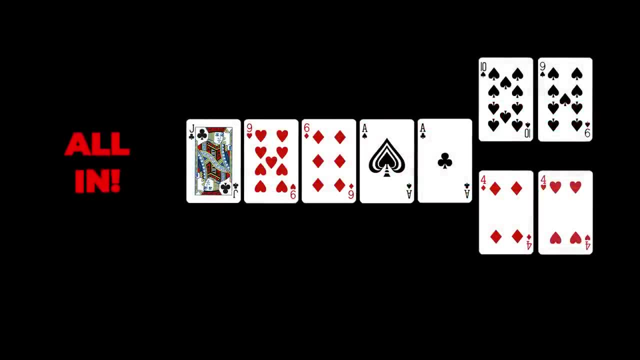 removal properties, For example. facing an all-in shove for our tournament life, we may decide to call with pocket fours but fold with ten nine, because holding the ten reduces the probability that villain is holding a bluff like ten, seven, ten, eight, queen ten or king ten, for example. 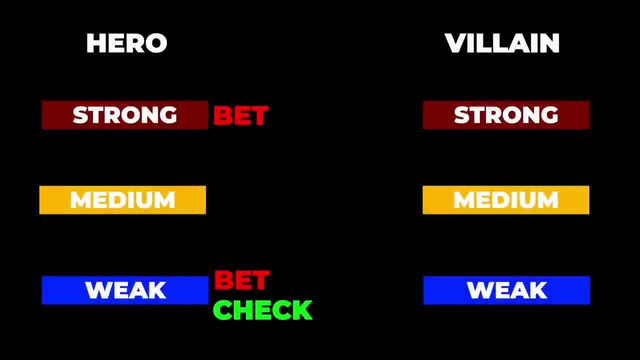 So, now that we've talked about what hero should do with his strong and weak hands, what about his medium hands? Well, since hands in this category generally will have a decent, but not great chance to be ahead of villain, they generally do not want to play for a big pot. 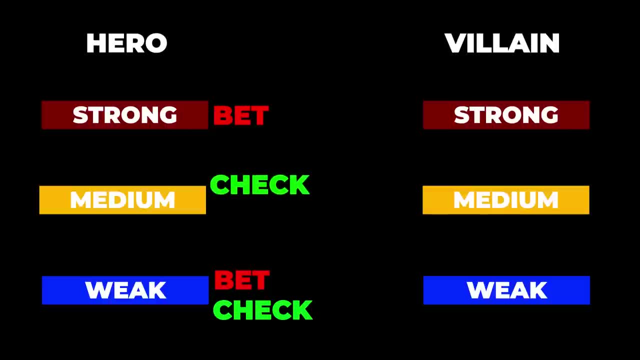 and will often be comfortable checking down and just scooping what went into the middle preflop. So these middling hands can often be played either way, as a bet or check, often depending on incremental equity. However, since we just mentioned that our strong hands usually want to bet over multiple streets, 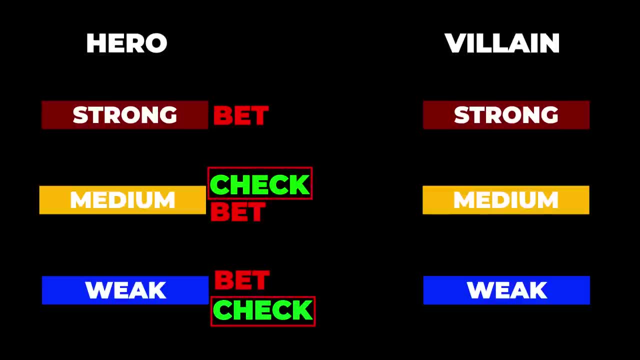 if we take a passive strategy, only with our medium hands and the weak hands that we give up. our discerning opponents would know that, when we check, the likelihood of us holding a strong hand is zero or very low, and he could leverage this information to apply maximum pressure against. 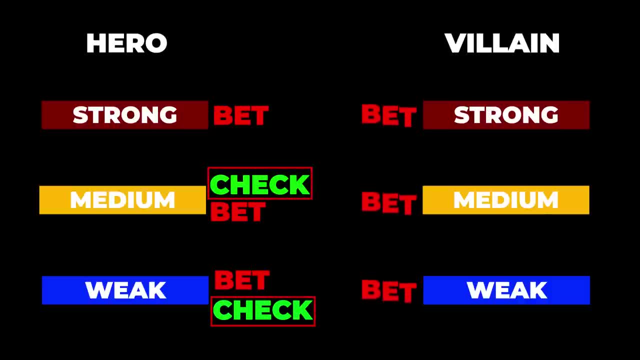 us making our lives miserable. So to protect our passive lines, we can start to also play passively with some of our strong hands, also known as slow playing or trapping, which sometimes also has the benefit of allowing our opponents to make a hand he likes on later. 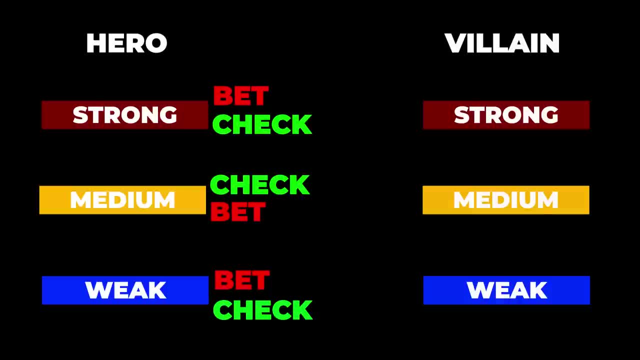 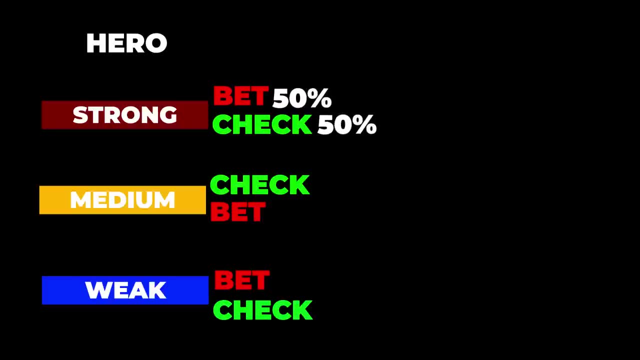 streets, whereas if we just bet, he might just fold. So how do we determine which strong hands to bet and which strong hands to slow play with? Again, we could just flip a coin, but even better, we could choose to slow play our hands, that one don't need much protection, and or two. 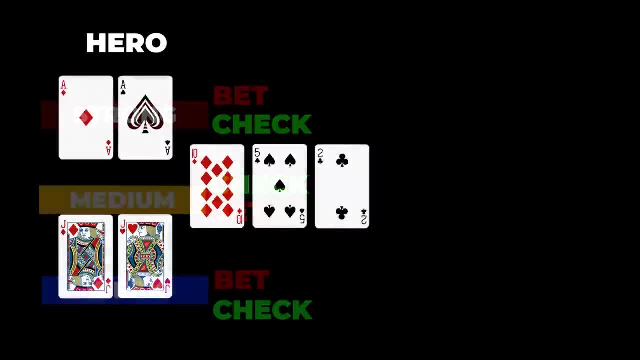 that block villain's calling range. So, for example, we may decide to cbet with pocket jacks but check pocket aces, because jacks could benefit from protection from overcards on turns and rivers, whereas aces do not need the same protection on this dry board. that villain. 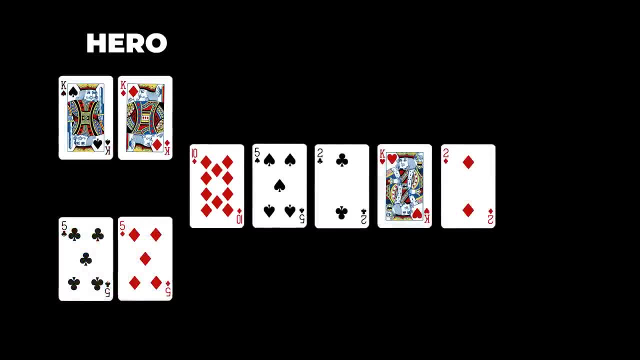 likely did not connect with, Or, in this river scenario, we may decide to slow play pocket kings but bet pocket fives, because holding two kings makes it much less likely that villain has top pair. or, in other words, our hand blocks top pair, which is a. 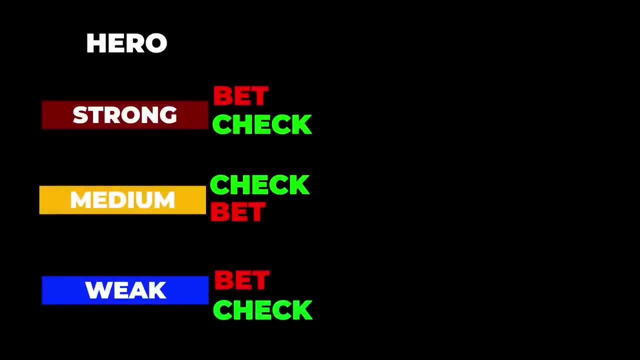 calling hand, whereas a pair of fives is not. And that is about it. What we've just described in a nutshell is essentially how every single GTO strategy is constructed. It doesn't matter if it's heads up, full ring, MTT or cash. GTO is mainly about maximizing our chips by balancing our strong. 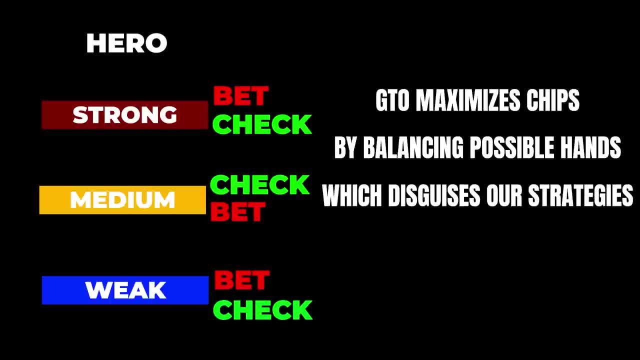 medium and weak hands in a way that makes our holdings and strategies very disguised and difficult, if not impossible, to take advantage of. And the key in terms of a practical application of GTO all comes down to combo selection, knowing which hands to fit within which bucket, depending. 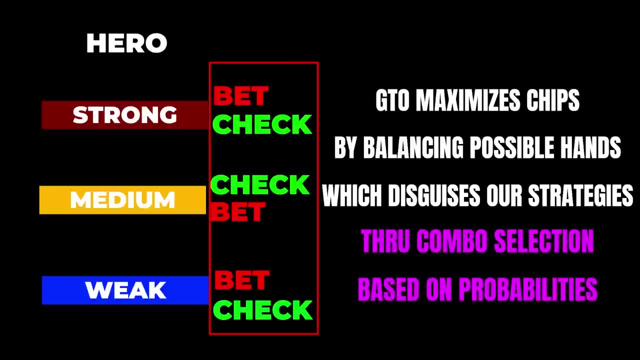 on its specific characteristics. But before we conclude this video, we should note a few caveats about GTO. First, notice how we discussed the need to balance our range in the context of facing a discerning opponent. In contrast, if your opponent 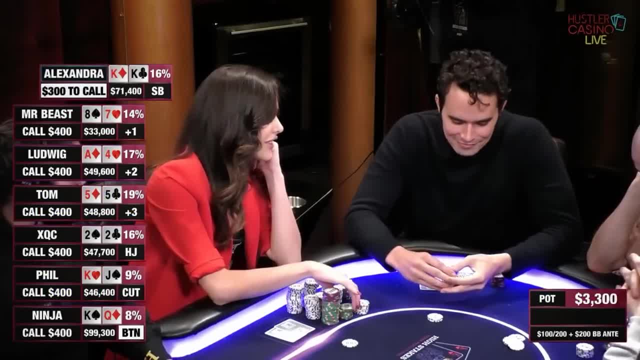 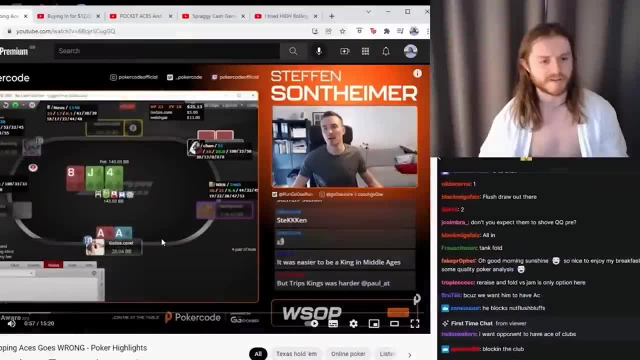 and not paying attention to what you're doing, then you can usually throw balance completely out the window, which is referred to as exploitative play. Second, even if your opponents are discerning, a practical real-life application of GTO doesn't require perfect balance. 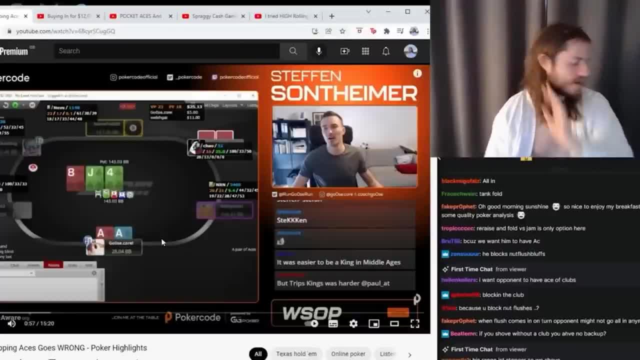 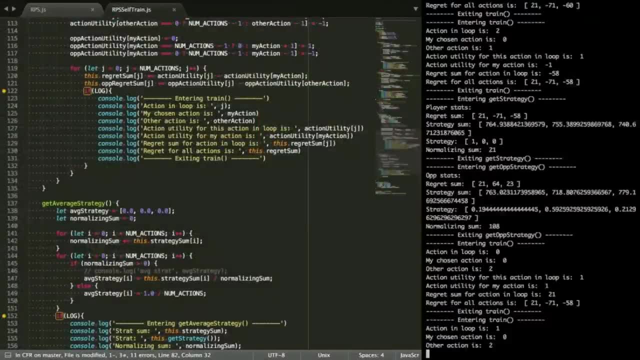 It requires just enough balance so that your strategies are not face up. Quote unquote: true GTO strategies are calculated by a computer playing a single hand against itself billions of times over, But in real life you aren't playing the same hand billions of times over. 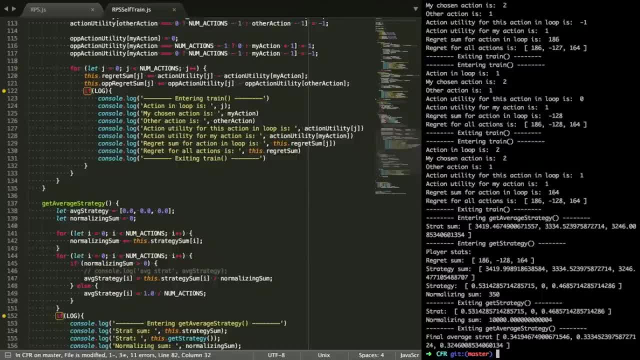 This means that even if you don't find balance in one particular hand, it probably won't matter as long as you maintain some semblance of balance over the long run. Additionally, when the computer plays against itself, it is clairvoyant, That is. 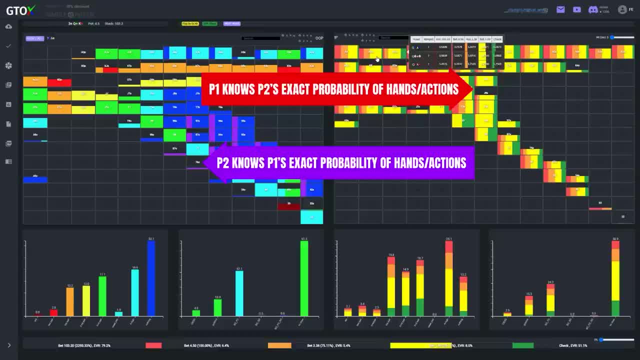 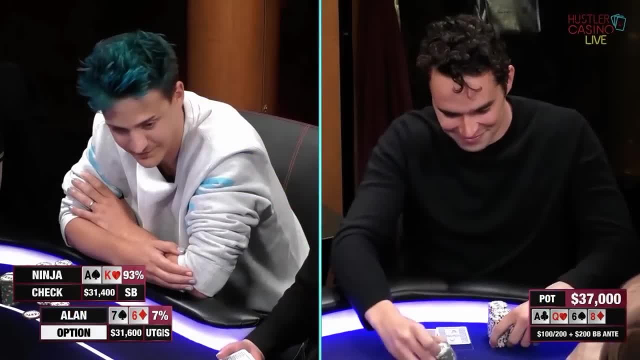 it knows the exact probability of hands its opponent can have and how frequently it takes each action. But your real-life opponents aren't clairvoyant. Some may not have even graduated high school, So you don't have to worry as much about maintaining. 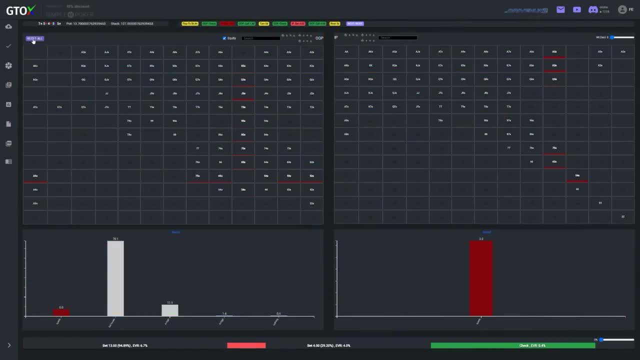 a perfectly balanced hand. This means that even if you don't find balance in one particular hand, it probably won't matter as long as you maintain some semblance of balance over the long run. And finally, although the overall premise of GTO is relatively simple and straightforward, 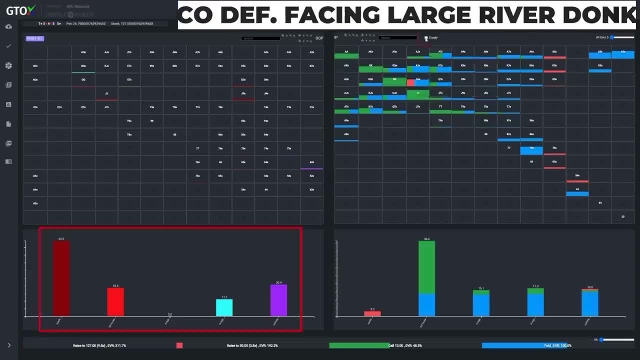 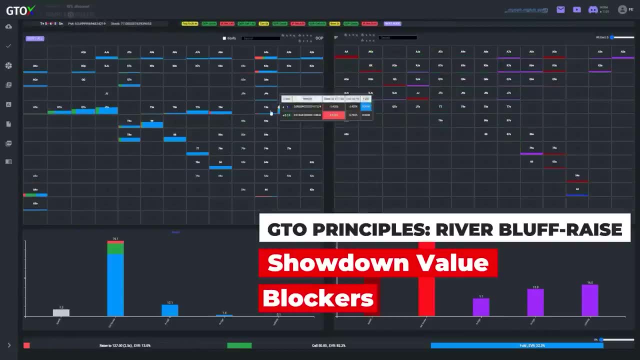 the execution of it is not. Knowing how to optimally balance your strategy can be incredibly difficult, as it will be impacted by numerous factors, such as the player's previous actions, board cards, the stack to pot ratio and position, and that's why you'll sometimes see: 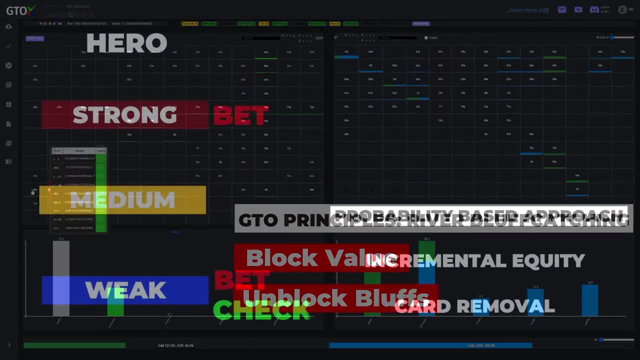 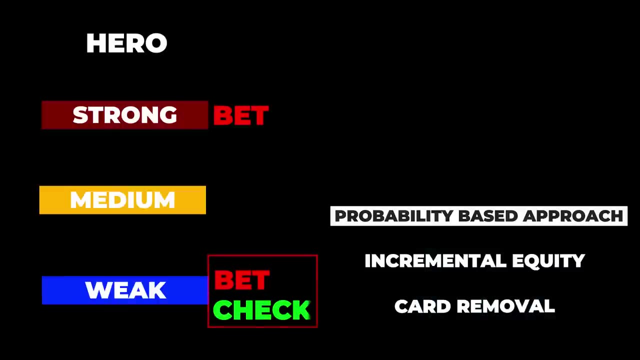 30 minute long videos going over a single hand on this channel. In this video, we only briefly touched upon how to rationally differentiate between the weak hands- we bluff- versus the weak hands- we give up, or the medium hands- we call versus fold, or the strong hands- we bet versus trap. 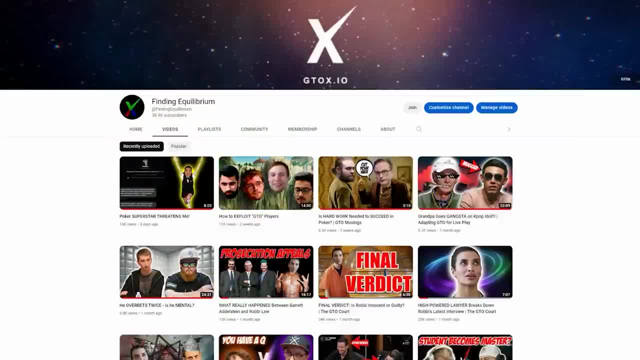 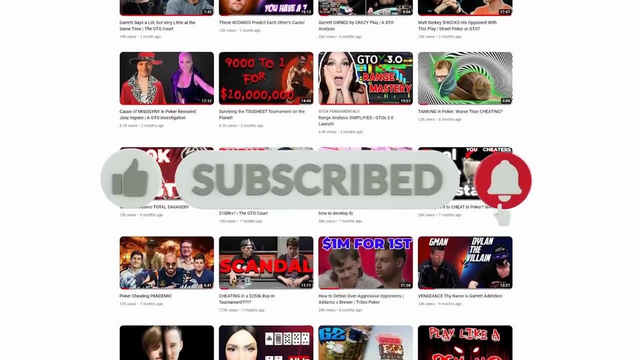 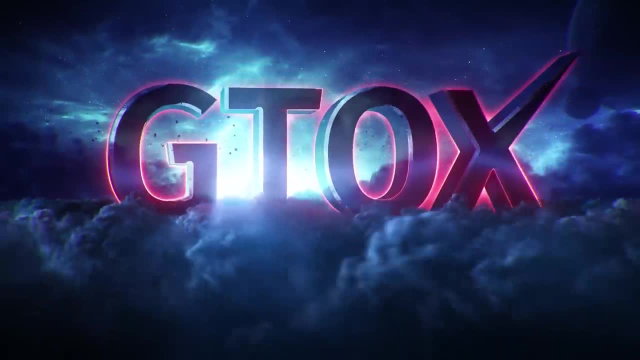 The reality is that there is a whole world of complexity that goes into making these decisions to maximize your edge. If you want to learn more about this world, hit that subscribe button and stay tuned for more videos. Thanks for watching. 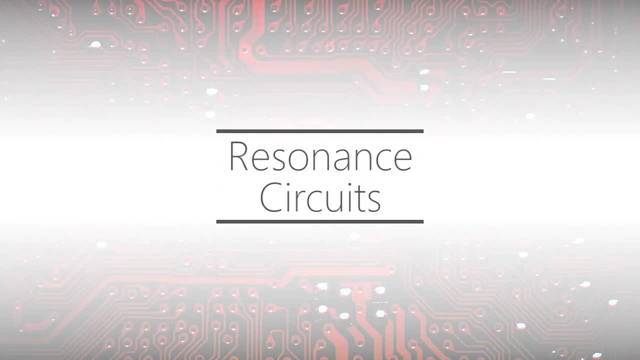 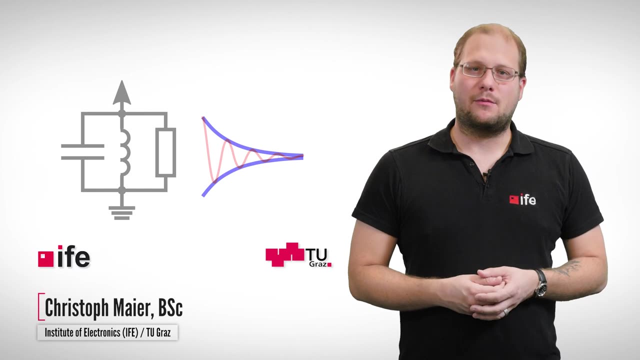 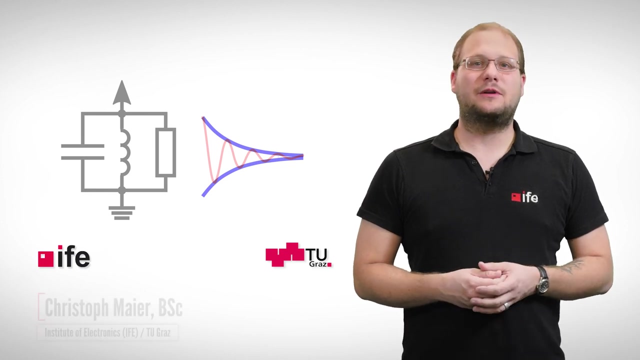 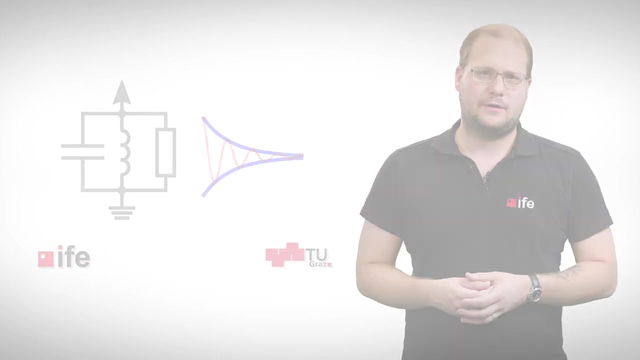 Resonance effects are practically everywhere in electronic circuits. Every time we have storage elements like inductors and capacitors, energy can be transferred between them. This can lead to effects that can make the life of an electrical engineer really difficult. In this video, we want to take a look at what is the root of resonances, how they cause.